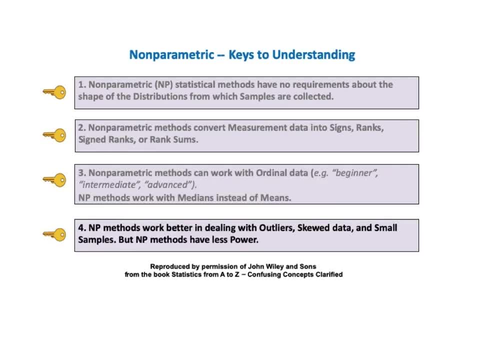 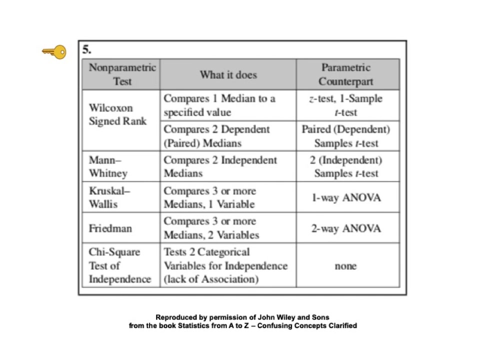 means Key to understanding. number four says NP methods work better than parametric methods in dealing with outliers, skewed data and small samples, but NP methods have less power. And the fifth key to understanding is this table of five common non-parametric tests, showing what each does and what its parametric counterpart is. 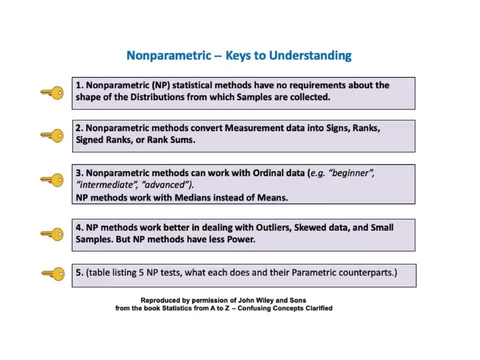 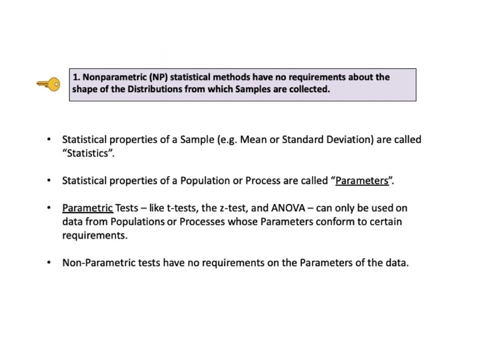 We'll go through this in detail, And here on one page are the five keys to understanding the concept of non-parametric. You may wish to pause the video at this point and read them all together. Okay, now let's take a closer look at each key to understanding. 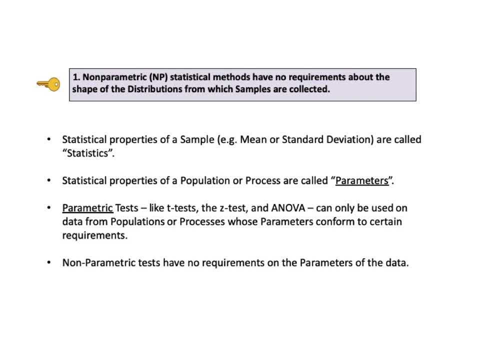 Key number one says: non-parametric NP. statistical methods have no requirements about the shape of the distributions from which samples are collected. Statistical properties of a sample, for example mean or standard deviation, are called statistics. Statistical properties of a population or process are called parameters. 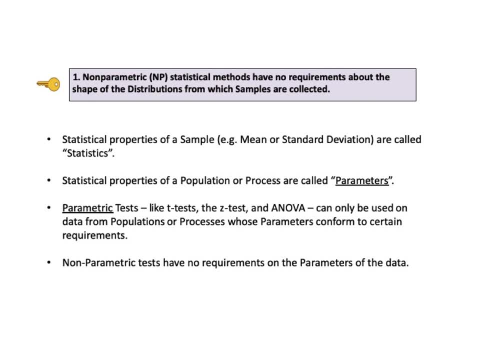 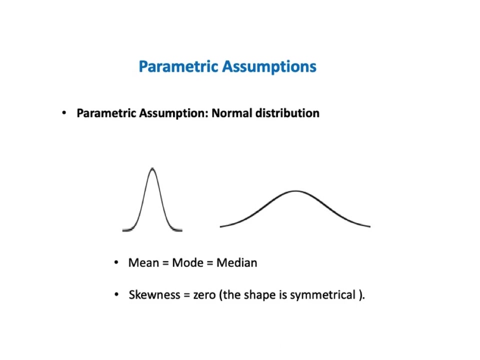 Parametric tests, like t-tests, the z-test ANOVA, can only be used on data from populations or processes whose parameters conform to certain requirements, but non-parametric tests have no requirements on the parameters of the data. The most common parametric assumption is that a population or process from which the sample 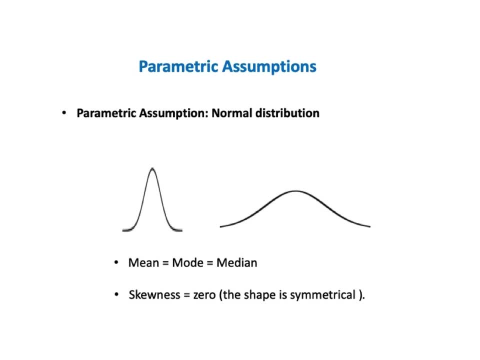 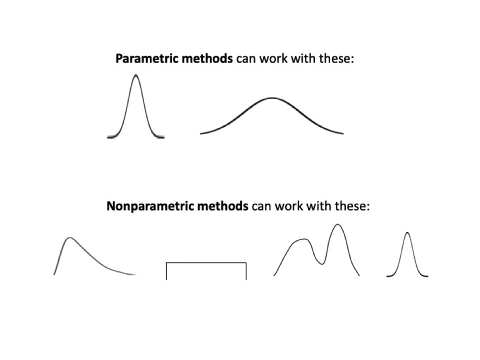 or symbols are drawn must have properties which are at least roughly normal. In distributions like those shown here, the mean equals the mode, which also equals a median, and the skewness equals zero. That is the shape is symmetrical. Non-parametric methods don't have those requirements on the data. 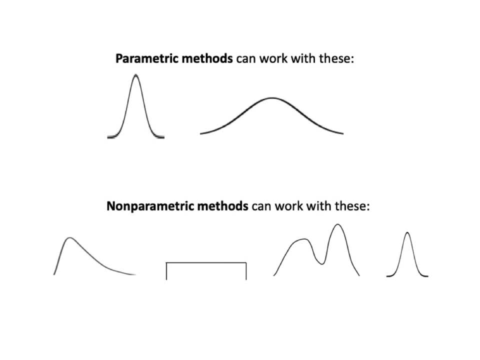 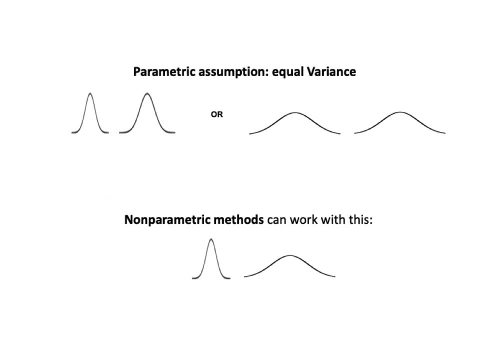 Non-parametrics can work with data on. numerically It doesn't matter how weird the shape of the distribution, even things like that shown here. Parametric methods which use two or more samples from two different populations or processes usually assume roughly equal variance. 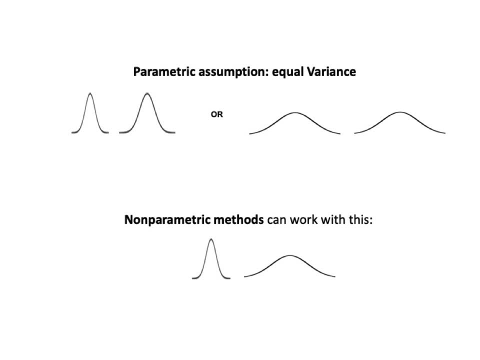 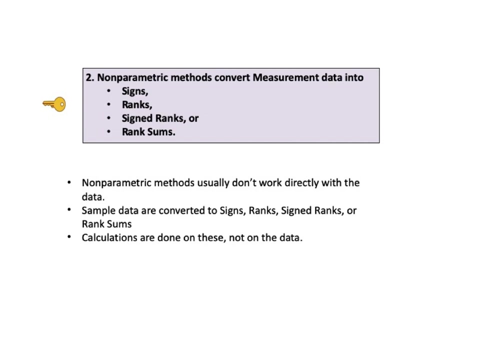 Non-parametric methods don't. Non-parametric methods are often called distribution-free because they are freed from any assumptions about the source distribution. Keto understanding number two says: non-parametric methods convert measurement data into signs, ranks, signed ranks or rank sums. 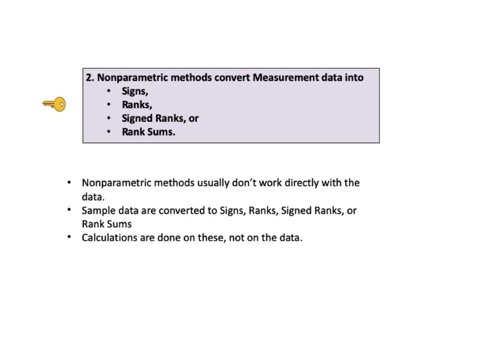 One reason that non-parametric methods can use data from any distribution is that they usually don't work directly with the data. The sample data are converted to signs and or ranks, as we'll soon see, and the numerical value of the data are lost before any calculations are done. 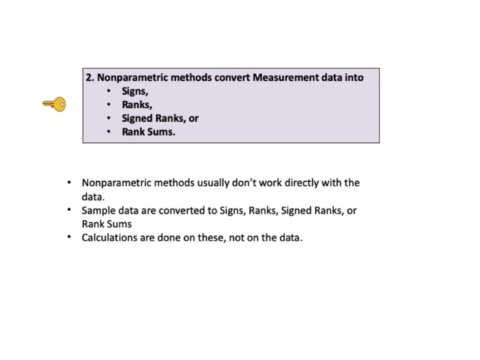 Calculations are done on the signs or ranks- or signed ranks or rank sums- not on the data. So it makes no difference what type of distribution the source data have. We're going to describe in detail how this is done in several non-parametric tests, but 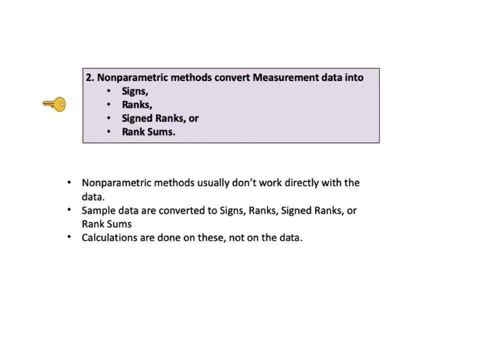 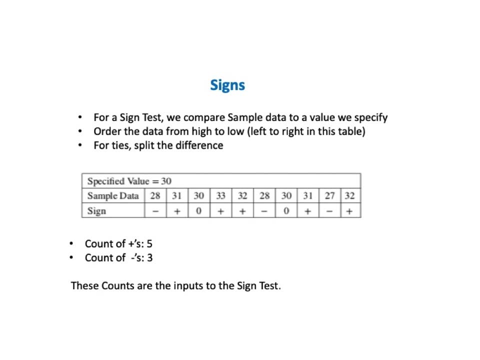 you don't have to do all this manually. Just enter the data into software for the appropriate test, Then it will do the rest. Here we have an example. using signs, We'll be comparing sample data to a value which we specify. That is what we do, for example, in a one-sample t-test. 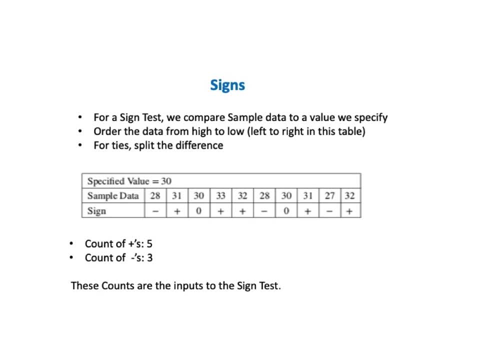 In this example, the value we specify is 30.. The specified value could be a target value or historical value or an industry standard, and so on. In this example, 30 seconds is a historical median time to complete an operation in an industrial process. 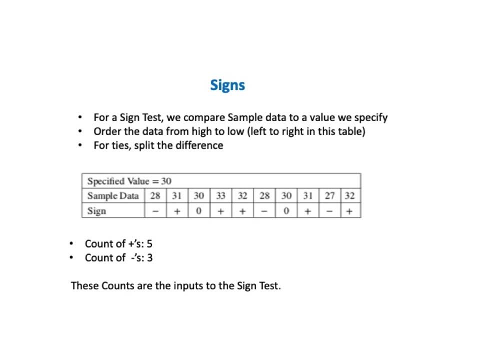 The second row shows the ten time measurements in seconds. in our sample, The values are 28,, 31,, 30,, 33,, etc. If a time is less than our historical median of 30 seconds, we get a negative sign. 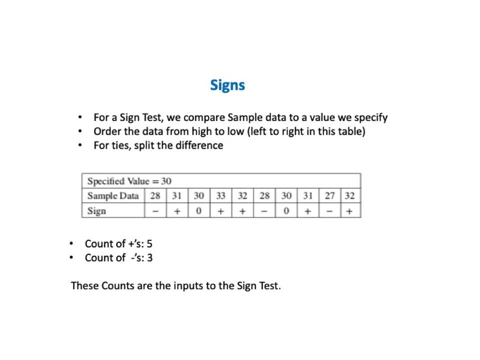 If it is equal to 30 seconds, it is a negative sign. seconds we give it a 0.. If it is greater than that median of 30 seconds, we give it a plus sign. Next we count the number of pluses and minuses. There are 5 pluses and 3 minuses. 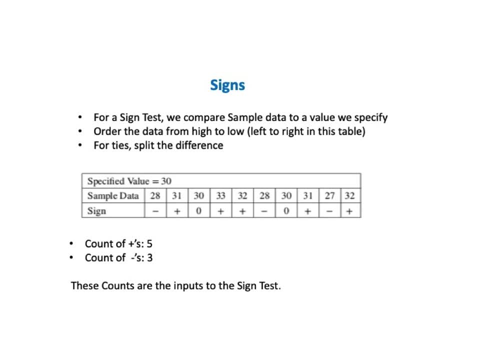 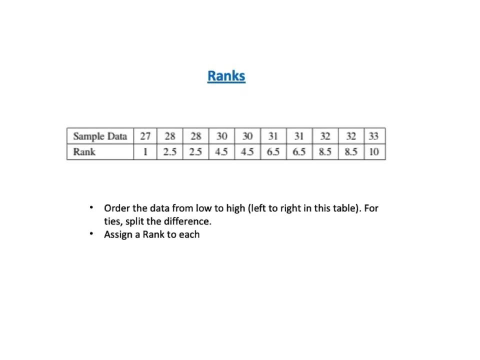 We can now use these counts instead of the original data in a nonparametric method called the sign test. Ok, that's how signs work. Now here's how ranks are used. Let's take the same sample of data and order it from low to high as shown here. Next, assign a rank. 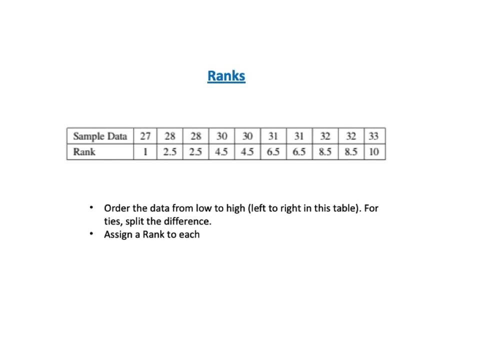 from low to high. The sample with the count of 27 is the smallest, so we'll give it a rank of 1.. For ties, split the difference between the values tied. For example, there are two 28s. These occupy the two ranks after a 2 and a 3, so we give them both a 2.5. 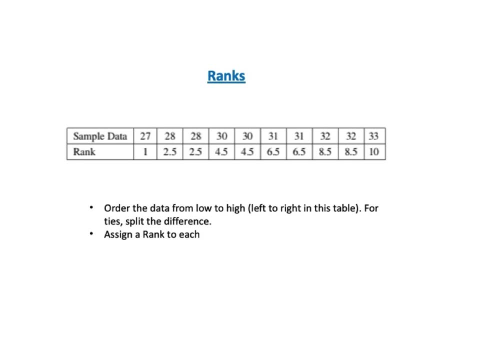 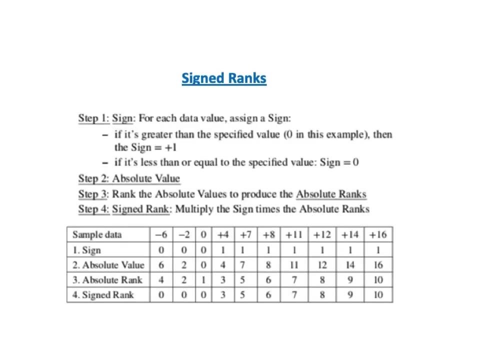 The next rank would be a 4,, but there's another tie, so we mark the next two as 4.5s, and so on. Signed ranks, as you might guess, combine the concepts of signs and ranks, But there is a change in how signs are assigned and absolute values are used. 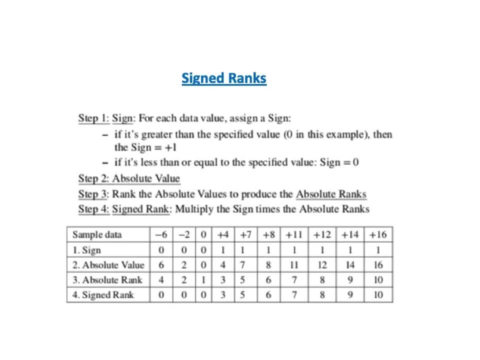 so we'll use a different example with some negative numbers. Let's say we are doing an analysis of the effect of a training program on employee productivity. If we were doing a parametric test, we'd use the paired t-test, which is also known as the dependent samples t-test. 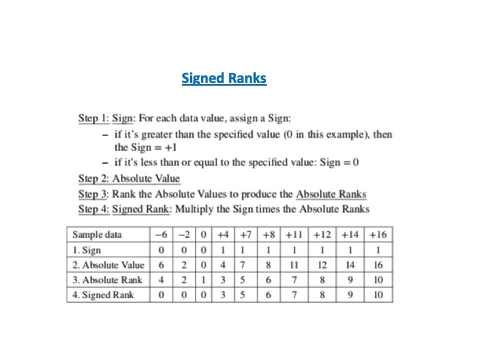 We count the number of transactions that the employees complete in an hour. For each employee, we subtract their score before training from their score after training. The data we are capturing is the difference. Instead of a plus and minus signs, we'll use plus one and zero. 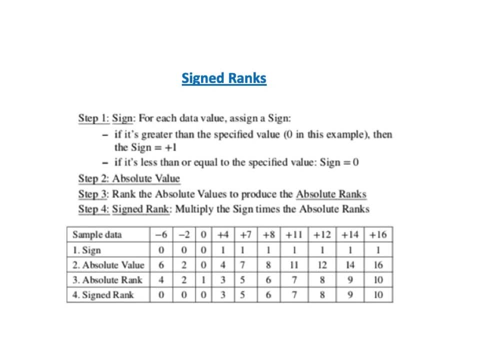 We compare the data values to a specified value, as we did in our example of a historical median of 30.. Each sample data value is their after-production number minus their before number. We'll be testing a null hypothesis, that there is a zero difference, so the specified value is zero. 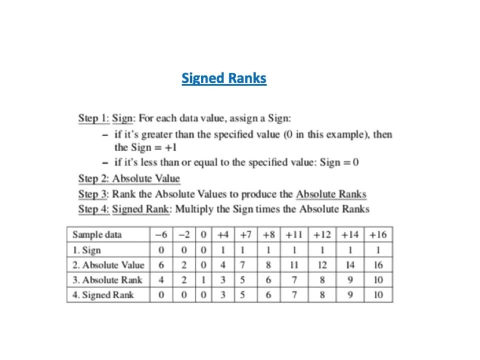 Step one sign For each data value assigned. if the sign is greater than a specified value, which is zero in this example, then the sign equals plus one. If it's less than or equal to the specified value, then the sign equals zero. 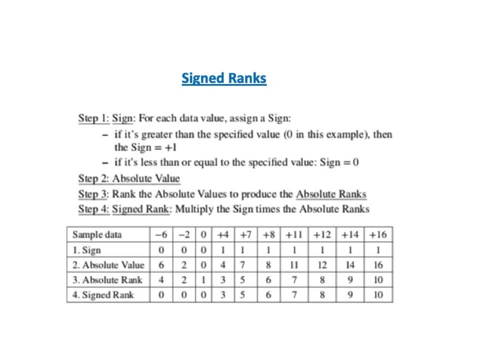 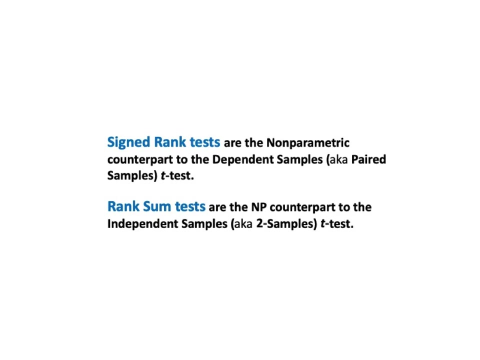 Step two is the absolute value. For step three, rank the absolute values to produce the absolute ranks. Step four: signed ranks. Multiply the sign times the absolute ranks. Signed rank tests are the nonparametric counterpart to the dependent samples t-test. 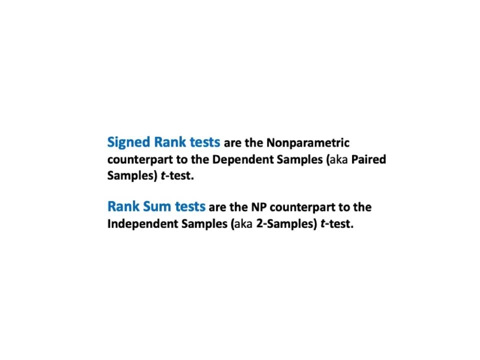 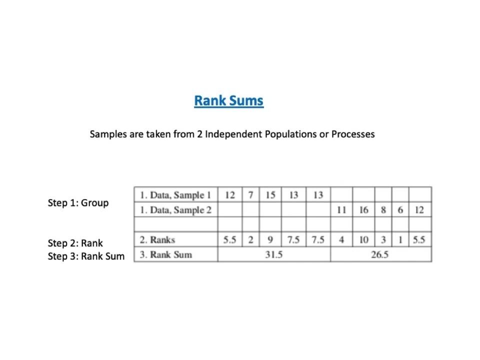 which is also known as the paired samples t-tests. Rank-sum tests are the nonparametric counterpart to the independent samples, aka two samples- t-test. Now let's take a look at rank-sum tests. We are comparing samples taken from two different analysis, such as Microsoft Y shares. 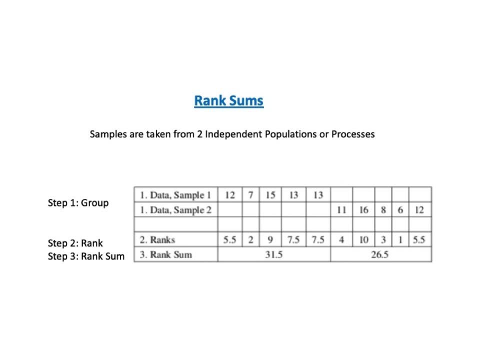 We are comparing samples taken from two independent populations of processes, That is, the data values of one population are not influenced by the data values of another. Step one group. Put all the data from both samples into a single group, but keep track of which ones came from which group. 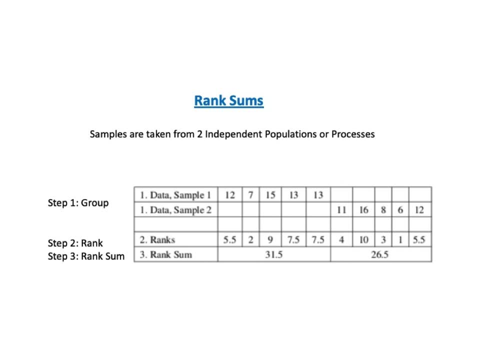 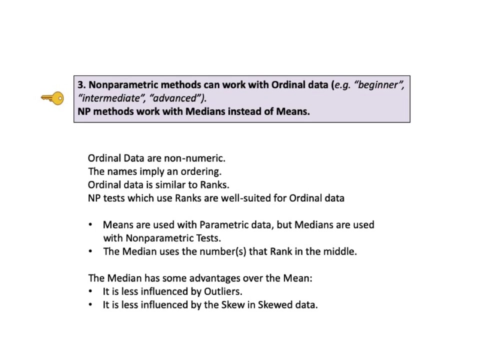 Step two rank Rank the values in the combined group And step three rank some Total the ranks for each sample Key to understanding. number three says nonparametric methods can work with ordinal data, For example, beginner, intermediate, advanced. 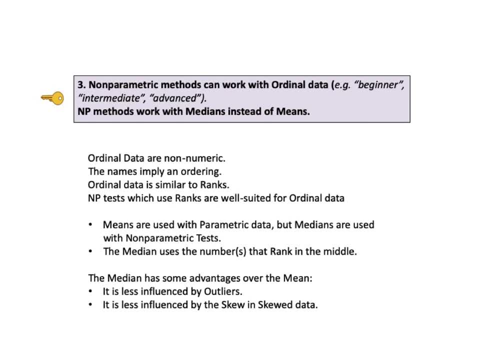 And nonparametric methods work with medians instead of means. Original data are non-numerical, They consist- I'm sorry, ordinal data are non-numerical. They consist of names and they imply an ordering, Hence ordinal, For example, beginner, intermediate and advanced. 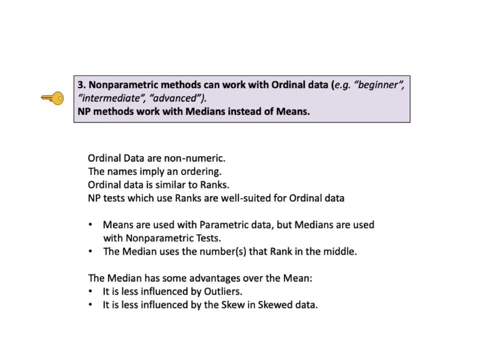 Or very bad, bad, neutral, good and very good. The names imply an ordering, but there are no corresponding numerical values upon which any calculations can be performed, Even if the names include numbers, for example moving ratings of one star to four stars. 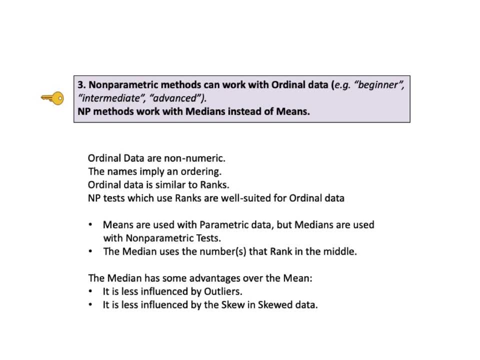 those numbers cannot be used in calculations. A four star movie is not defined as 1.33 times one. The order in ordinal data is similar to the ranks in nonparametric NP statistics, So NP tests which use ranks are well suited for ordinal data. 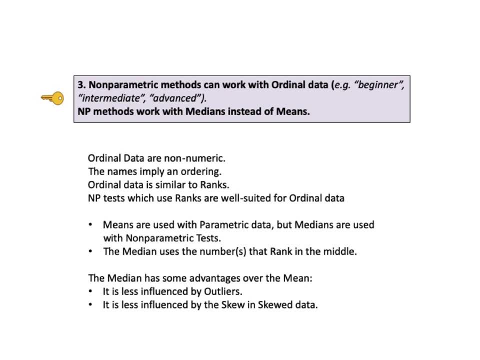 Means are normally used as a measure of central tendency in parametric tests. In converting the data to signs, ranks, etc. we lose the ability to calculate the mean, So we use the median instead. The median is another measure of central tendency. 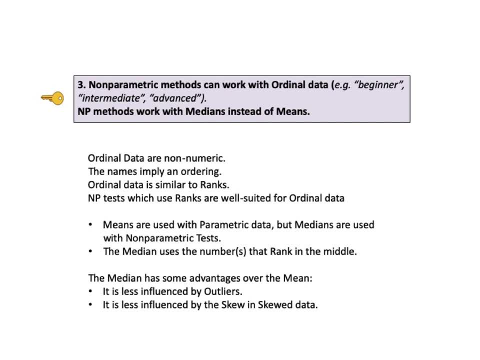 It is well suited for NP tests because it uses the numbers that rank in the middle To determine the median. arrange the data values in order low to high or high to low. For an odd number of data values, the median will be the middle value. 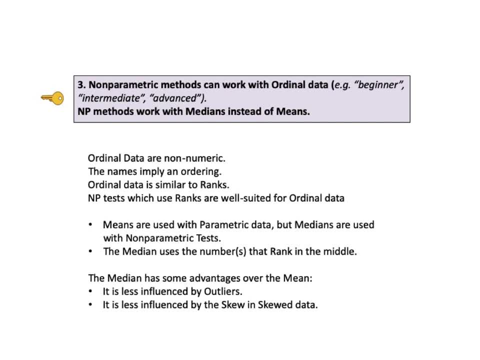 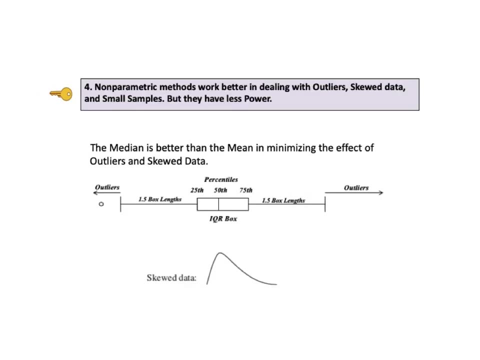 For an even number, it will be the average of the two middle values. The median has some advantages over the mean: It is less influenced by outliers And it is less influenced by the skew in skewed data. KTU number four says Nonparametric methods work better in dealing with outliers, skewed data and small samples. 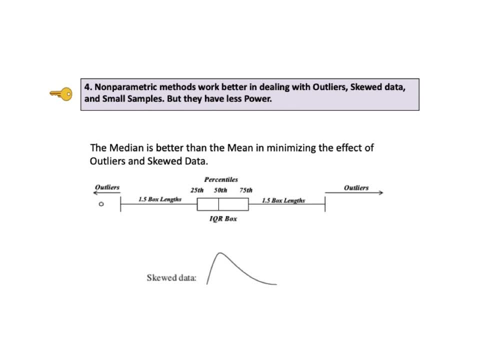 But nonparametric methods have less power. Since nonparametric NP methods use the median instead of the mean, they are better than parametric methods in minimizing the influence of outliers and skewed data. For that reason, in certain situations the median is a more useful measure of central tendency than the mean. 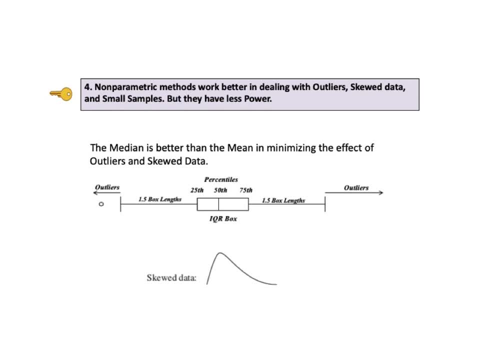 Here is an example: A couple is looking for a house in a community in which most houses are in the price range they can afford, Say $400,000.. They look at a report on recent home sales which show mean prices. One community shows a mean price of about $670,000. 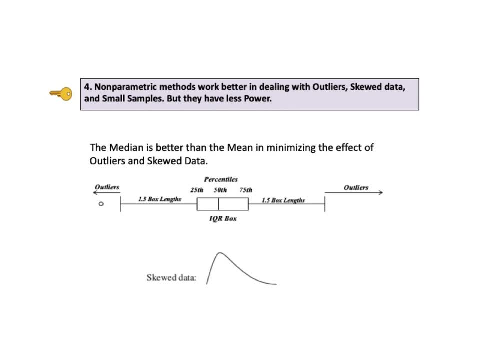 So they immediately exclude it from consideration. However, the underlying data show that five houses were sold for around $400,000 and one outlier was sold for $2 million. The median for the same numbers would be around $400,000.. Just what the couple was looking for. 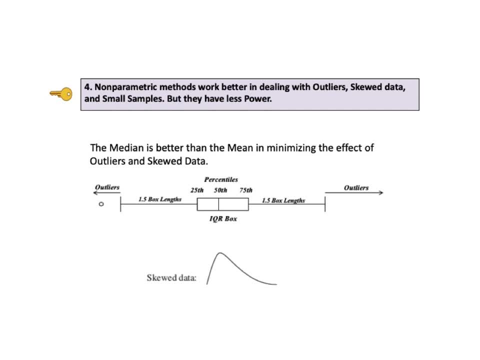 Similarly for skewed data, the mean can be a less meaningful measure in a practical sense than the median. Of course, with skewed data the assumption of normality would not be met, So an NP method would need to be used in any event. 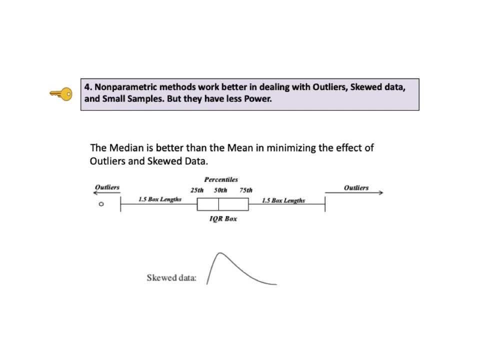 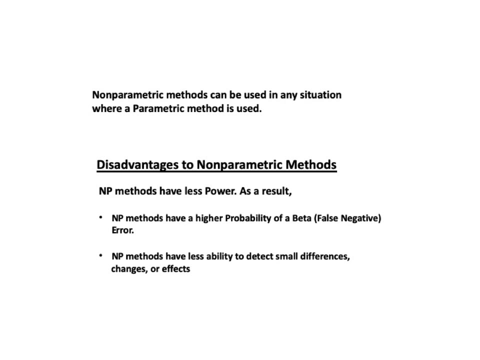 For small sample sizes it is not possible to accurately determine whether the distribution is normal. So a small sample size is a reason to use the NP method. Nonparametric methods can be used in any situation where a parametric method is used. The opposite is of course not true. 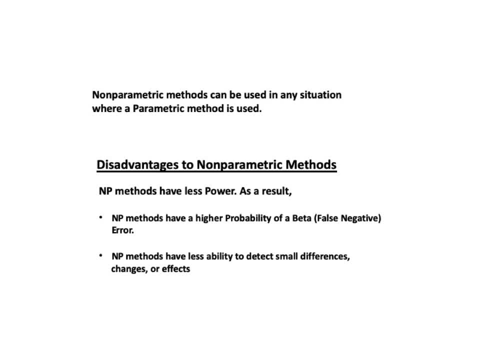 So why wouldn't you use NP methods all the time? Well, NP methods have less power. This means that NP methods have a higher probability of a beta error, which is also known as a false negative error. NP methods have less ability to detect small differences. 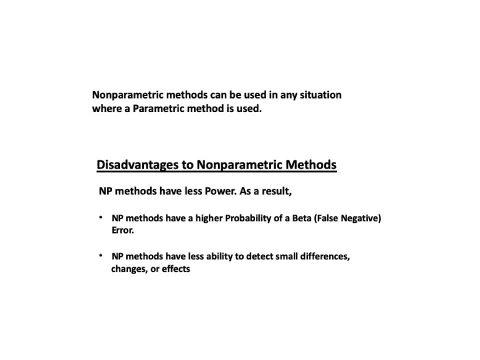 changes or effects. A beta error is a false negative error and beta is the probability of a beta error. Power equals 1 minus beta. It is the probability of not having a beta error, the probability of not having a false negative error. 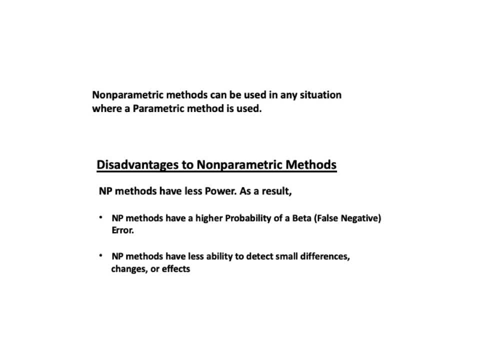 Lower power means that NP methods have a higher probability of beta error or false negative error than parametric methods. Also, lower power means a larger minimum effect size. Now, why is this the case, When nonparametric methods convert from measurement data to signs and ranks, for example? 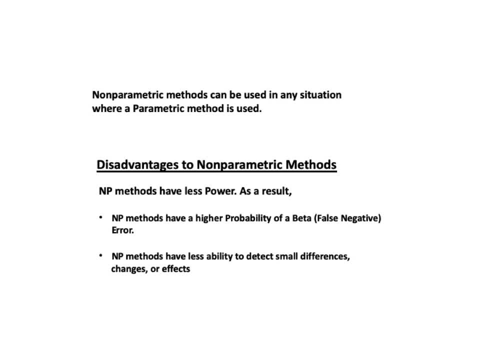 information, and thus precision, is lost. The 3rd and 4th ranked measurements in the data may be 25 and 26,, while the 9th and 10th ranked numbers may be 35 and 45. Ranks and signs would lose the information. 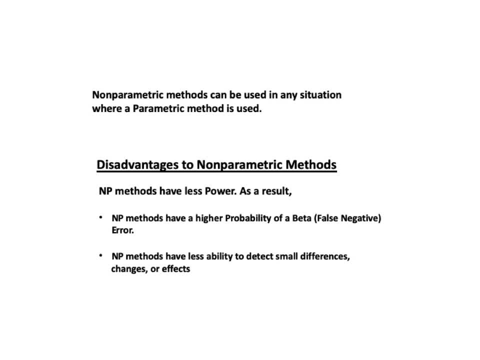 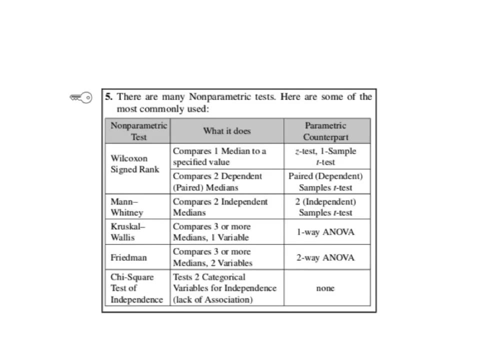 that the difference between the 9th and the 10th ranked numbers is 10 times as much As the difference between the 3rd and 4th. This reduction in precision is what causes the power of the test to be reduced in NP methods. 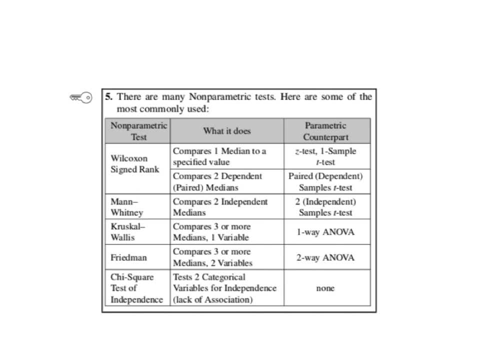 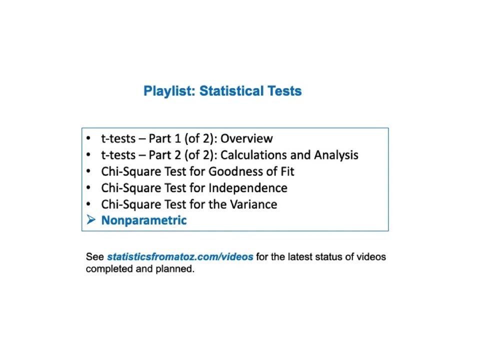 Keto understanding number 5.. There are many nonparametric tests. This table shows some of the most common ones and what their parametric counterparts are. You may wish to pause the video to read them. That concludes our discussion of the nonparametric tests.